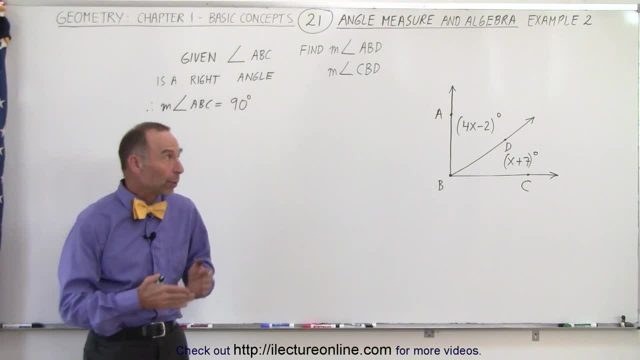 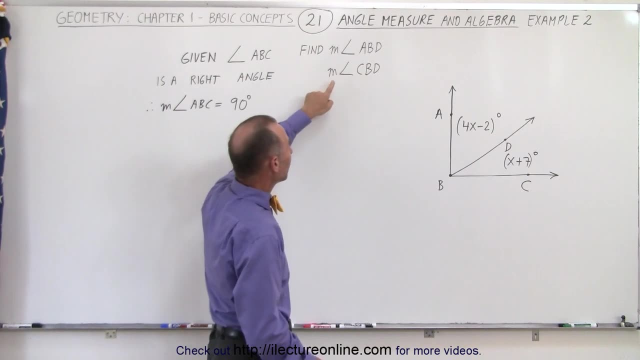 Welcome to our lecture online. Here we have a second example where we're trying to figure out the measure of the two angles indicated. We're trying to find the measure of the angle ABD and the measure of the angle CBD. We're told that the angle ABC is a right angle, so the angle from 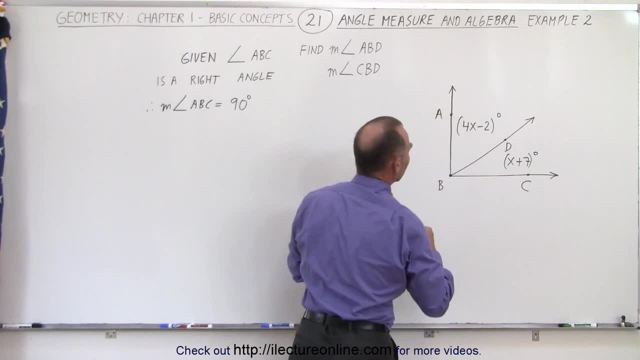 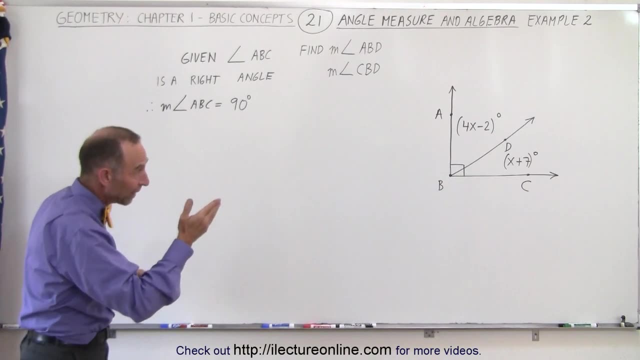 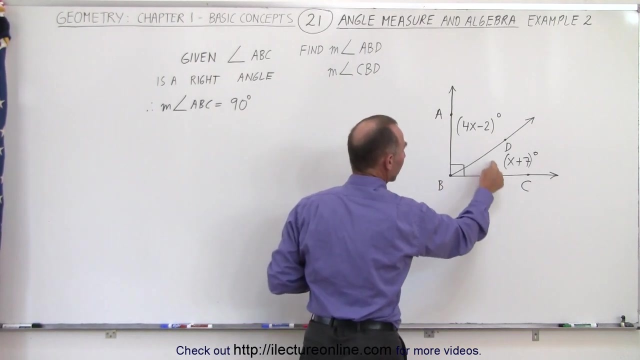 ABC between these two rays. that angle here is the right angle, so we can indicate that by drawing these. that means that the angle of ABC has a measure of 90 degrees, which means that the angles measures of these two angles must add up to 90 degrees as well. so therefore we can say that 4x. 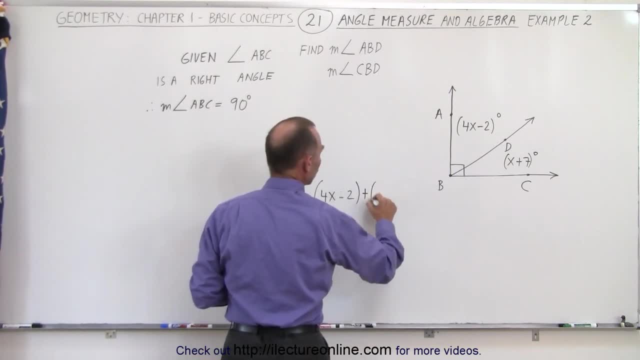 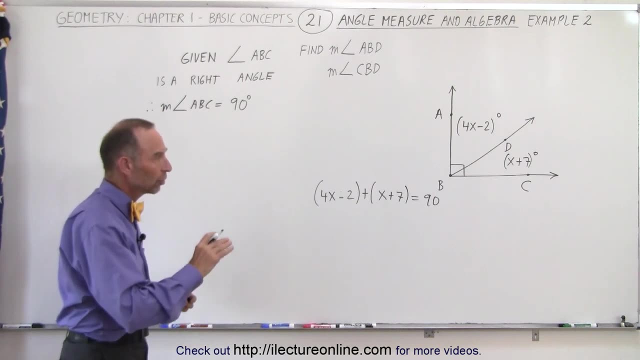 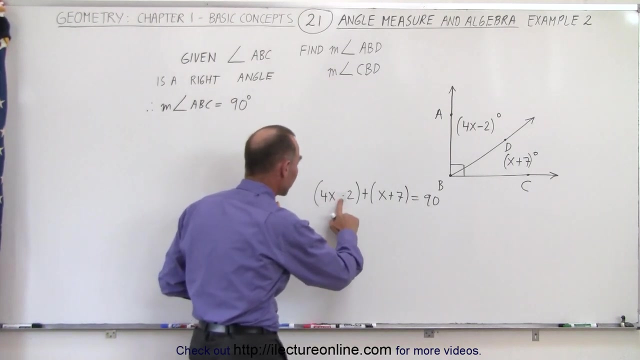 plus 2 added to x, plus 7 must add up to 90. Here I simply ignored the degrees, because it makes it easier to work out the problem. What we're going to do now is find the value, and oh, I made a mistake here. this should be for x. 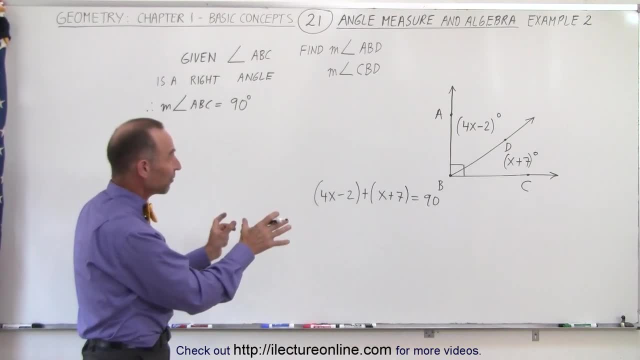 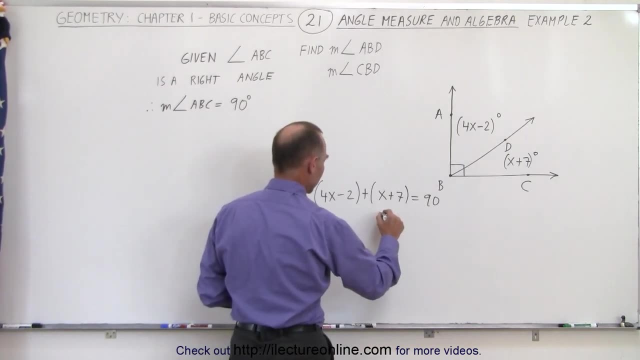 minus 2, and so what we're going to do now is find the value for x and then calculate the measures of the two angles. So combining all the x's on the left side we end up with 5x is equal to 90, the 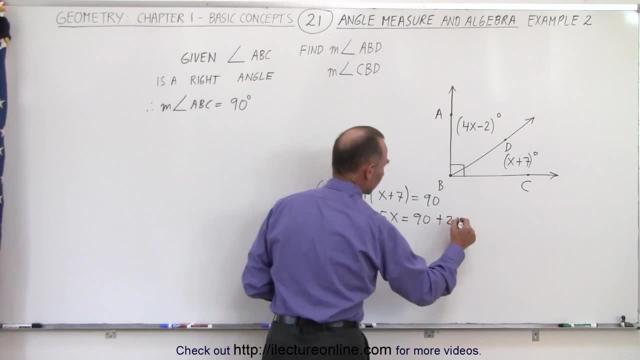 minus 2 goes across becomes plus 2, and the plus 7 goes across becomes minus 7, which means that 5x is equal to 85. divided by 2, x minus 7 is equal to 95.. for both sides by 5, we get X is equal to 17. so now, given that we can find the 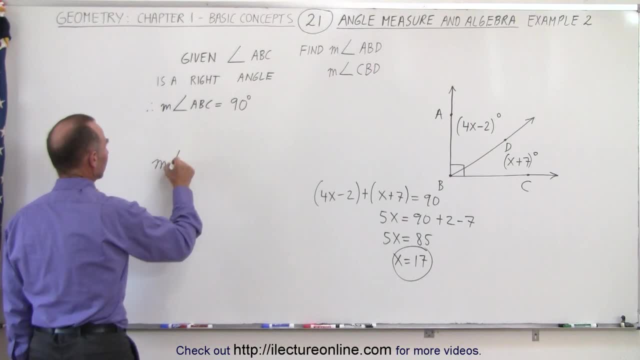 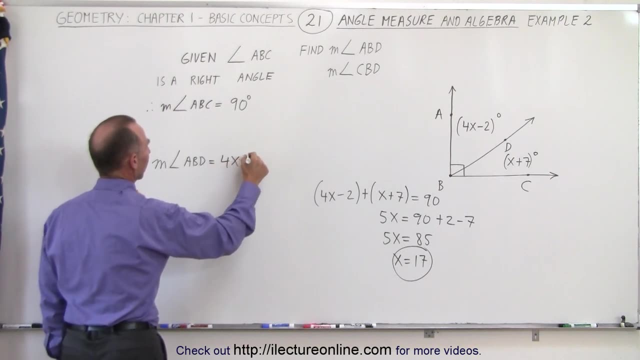 measure of the angle ABD. the measure of the angle ABD is equal to 4x minus 2 degrees, and since X is equal to 17, that is equal to 4 times 17 minus 2. put parentheses around it: degrees 4 times 17, that's 68 minus 2, which is equal to 66. 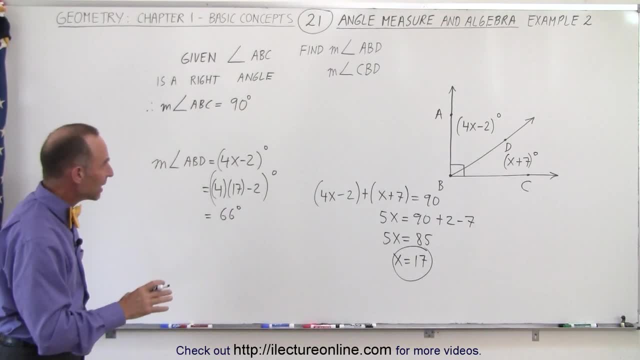 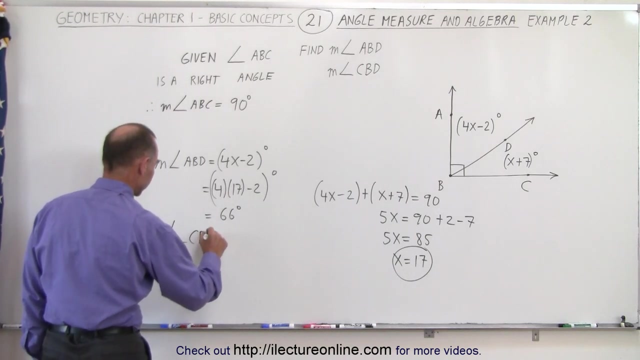 degrees. so the measure of the angle ABD is 66 degrees, which means that the other angle should be 24 degrees. 66 plus 24 is 90, but let's work it out and see. so the measure of the angle CBD is equal to X plus 7, and that would be degrees of.